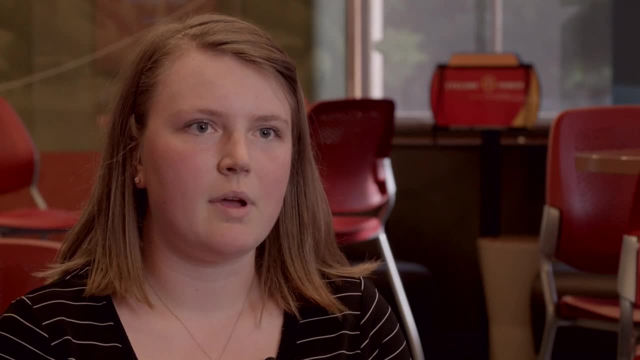 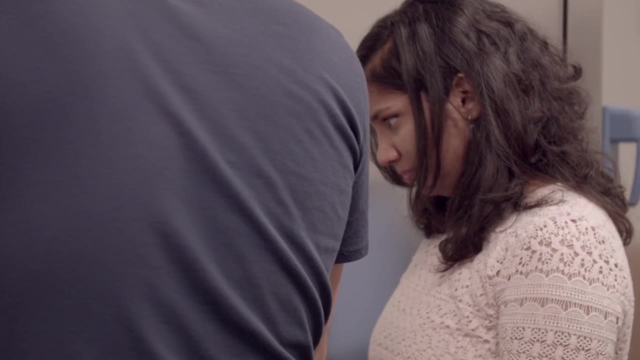 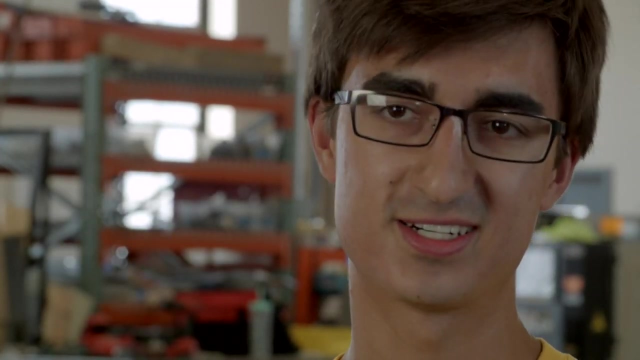 saying: how can we make this material better in order to help our device function better? We create, innovate, transform, optimize how these materials work. Materials engineers: just take all materials, make them stronger, lighter, faster, making easier to process biodegradable. What? 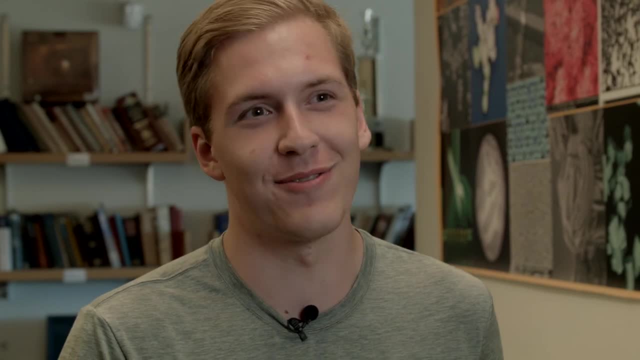 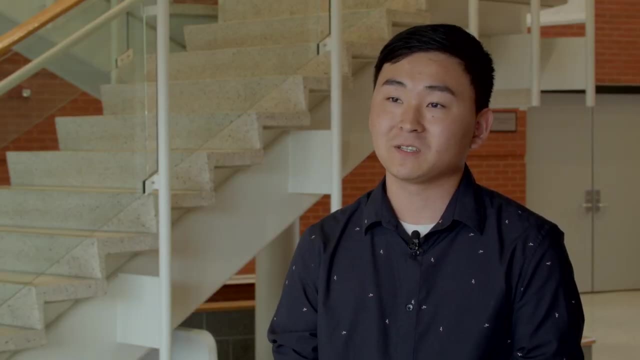 makes it exciting is: it's a new technology. It's a new technology. It's a new technology. It's a newer field, especially with 21st century technology, we're able to start doing stuff like smart materials. It's always changing and you're always learning something new. We are still on that. 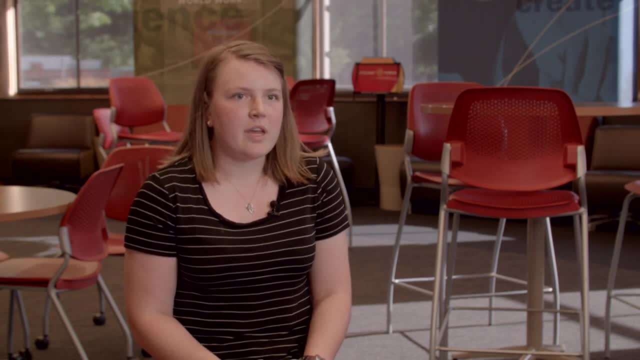 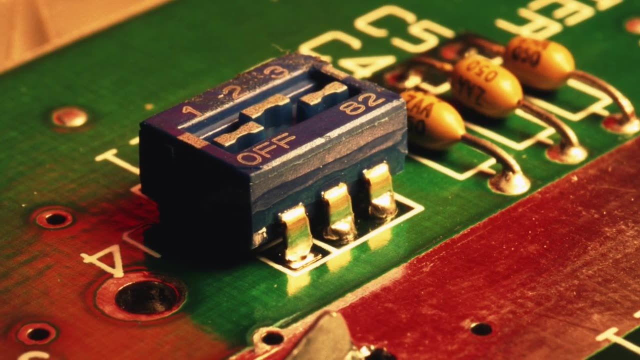 cutting edge, discovering completely brand new things. Typically, materials are what brings the next stage in a lot of technologies. Think about the bronze age or even silicon. Once we were able to make silicon wafers and stuff in high purity that ushered in computers and all sorts of that. 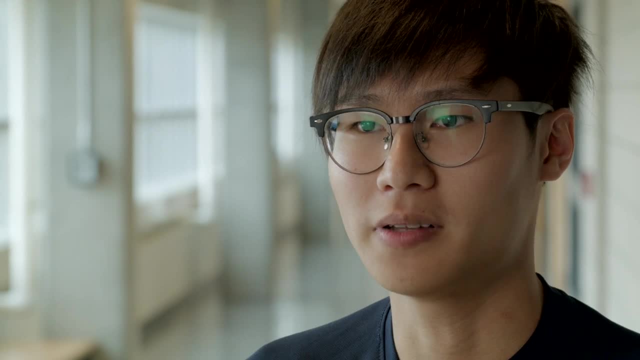 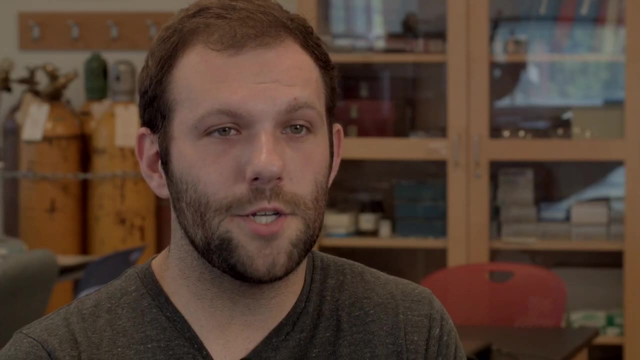 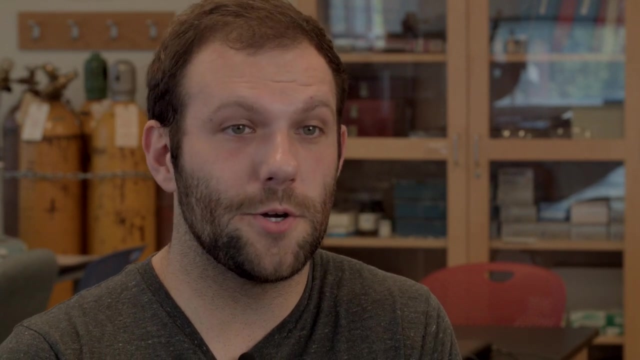 Material engineering is kind of relatively new field study compared to other engineering, so it has a lot to explore and learn. All the engineering problems that we deal with today are either limited by the design or the way that it's made or, ultimately, more so, the materials that we 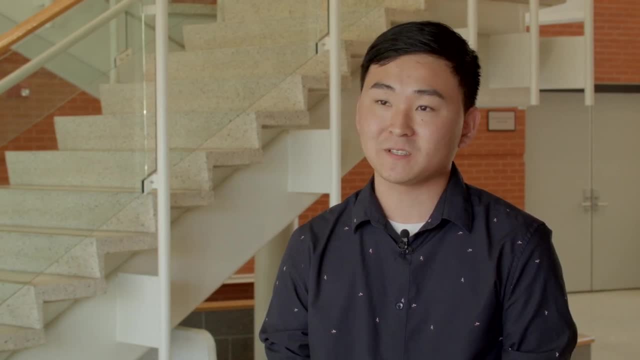 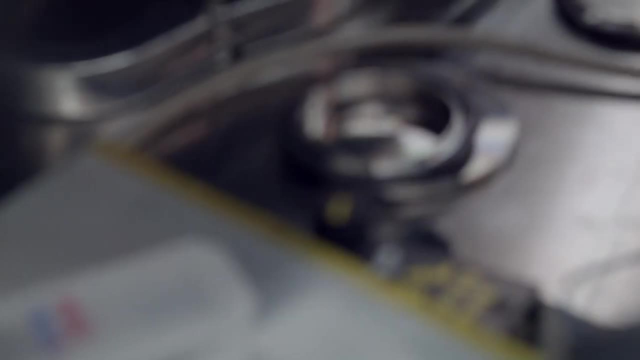 use. I chose- mainly chose- material science and engineering, again because it was diverse and there was a lot of different things you could work on. I really didn't think of my own career, future or about what I wanted to be literally. I really wanted to be a computer scientist and doing my 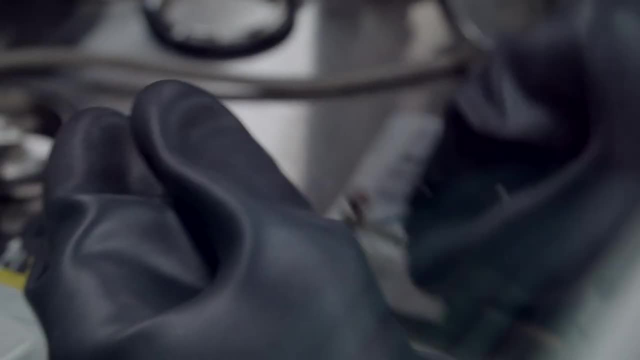 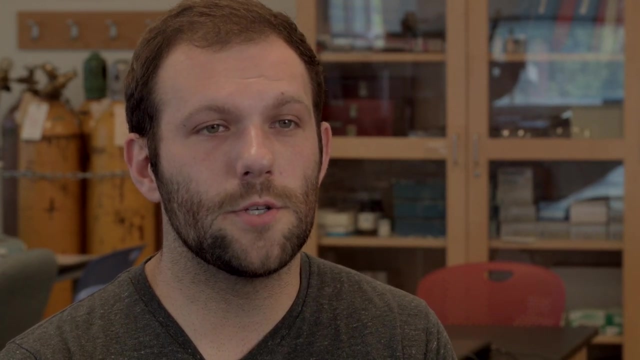 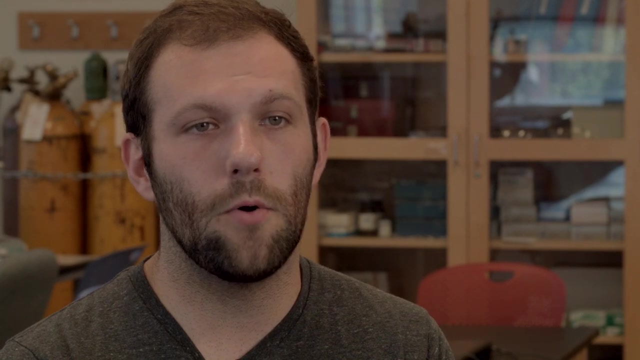 I just found this, this field that I is just incredibly interesting. Iowa State was the school I chose because the other schools I looked at that offered materials programs only really focused on one type of material, like metals or polymers or ceramics, but none of them covered the whole breadth that we do. 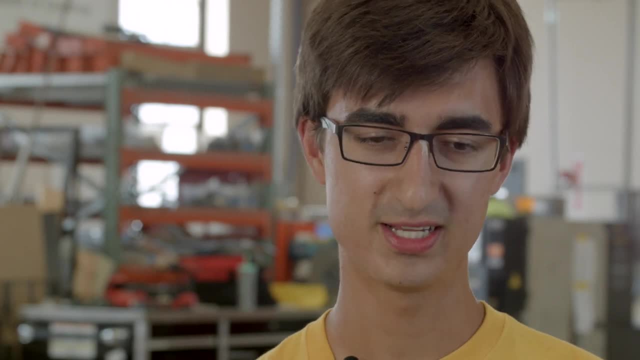 here at Iowa State. I had family in Iowa so I kind of heard about Iowa State and they've kind of been hinting to me like, hey, you should go here or something. so I decided to take a look at it. Turns out really good engineering school. I like to. 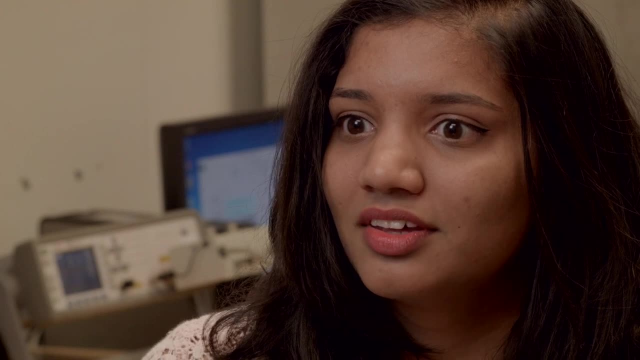 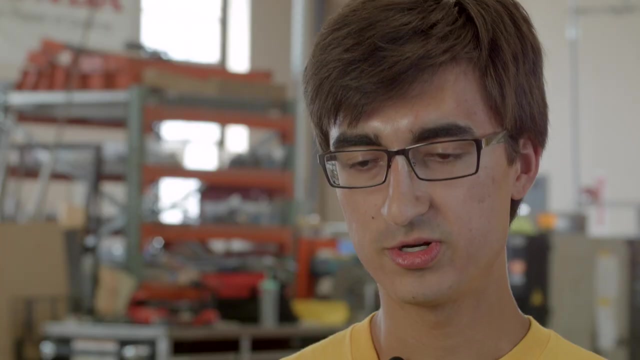 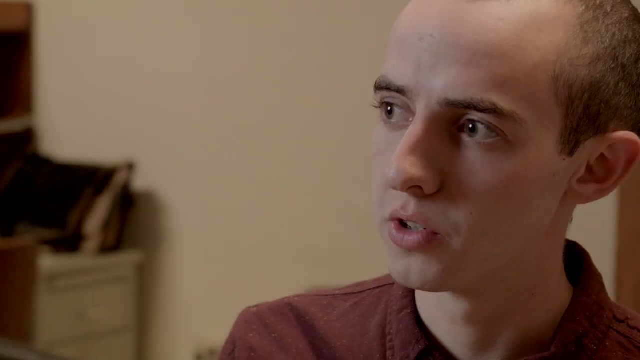 think of material science, as that discipline, that sort of gives me the diversity and flexibility to explore a lot of different fields in one place. My dream job would be doing research on some really interesting material that most people haven't really heard of, Because I would like to work in the